so I'm going to keep my numbers on the right. So I look right here and I see, hey, this is a negative 8x. so I'm going to keep my numbers on the right. So I look right here and I see, hey, this is a. 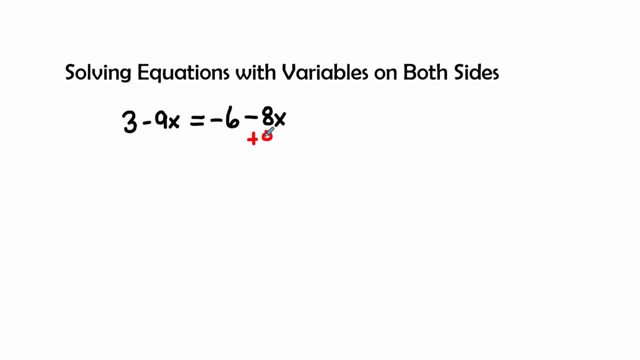 negative 8x. so the inverse of a negative 8x is a positive 8x. Now we're going to what we do on one side of the equation. we're going to do exactly on the same side of the equation to 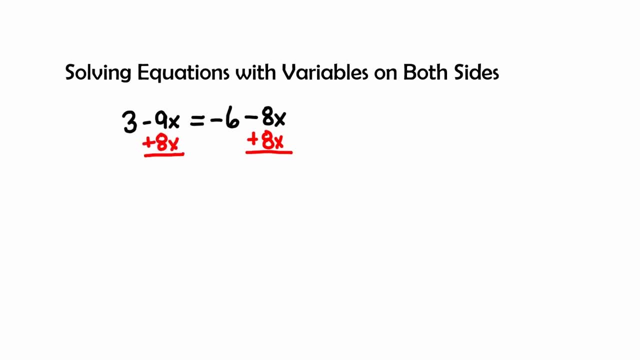 keep this equation balanced. So here we go. we're going to rewrite everything and simplify and combine. So we have 3 negative 9x plus 8x is a negative, x equals a negative 8x. So we have negative 6 and then a negative 8x, and a positive 8x gives me 0. So now I'm down to my next step. I 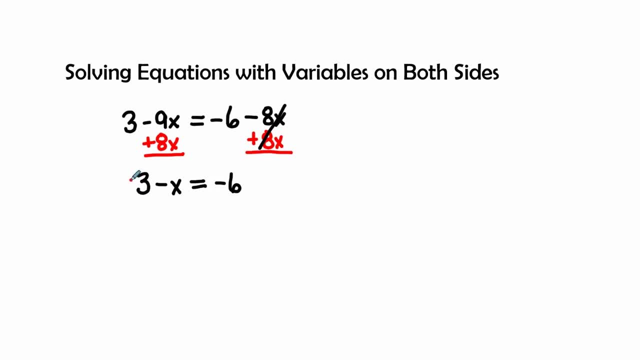 then see that I have my number or my number term, my constant term. that is a positive 3.. And with the inverse of a positive 3 is a negative 3.. So I'm going to add a negative 3 to both sides of 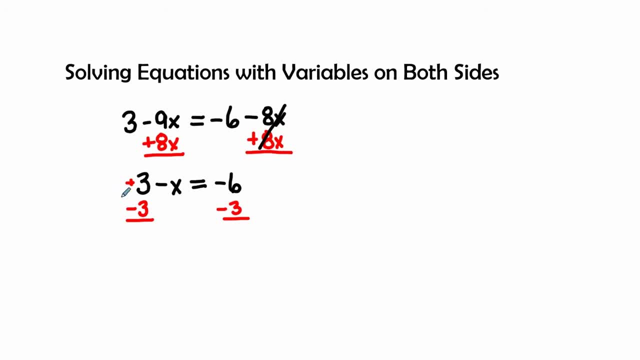 the equation. to keep it balanced, A positive 3 is a negative 3.. So I'm going to add a negative 3 and a negative 3 gives me 0. So I have a negative x equals negative 6 and a negative 3.. 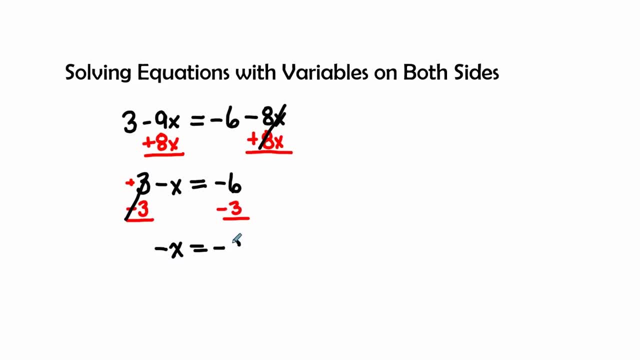 I combine those terms together, which will give me a negative 9.. Now I see that, well, I have my variable by itself, but not entirely. I have this negative x, so it's really kind of like a negative 1 here. So I need to divide the variable x by a negative 1.. 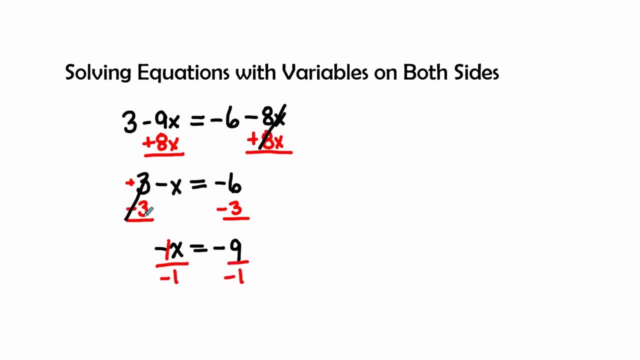 And then I can simplify, And so a negative 1 divided by a negative 1 gives me x Negative, 9 divided by a negative, 1, negative and a negative is a positive, and 9 divided by 1 is 9.. And so 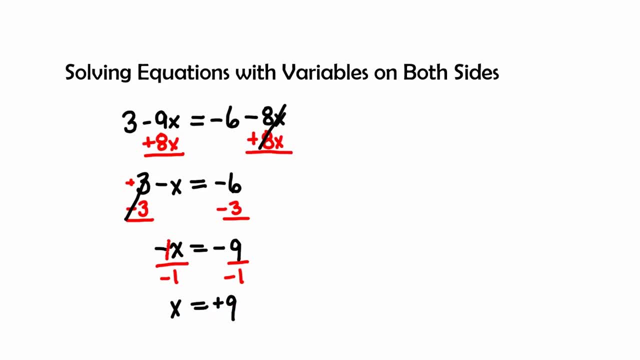 x equals a positive 9, is my answer. So let's go ahead and check my work. And so I have negative 3 minus 9.. And in place of the x, I'm going to put a parentheses. So I'm going to put. 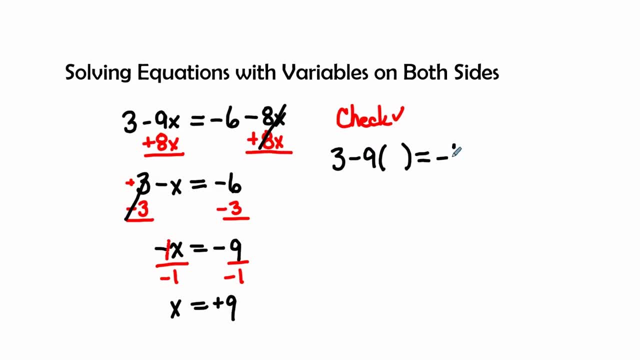 this positive 9 in Equals a negative 6 minus 8, open parentheses, close parentheses for that positive 9.. So I'm going to put my 9 here And I'm going to have a 9 there. So let's go ahead and bring everything down and simplify these. 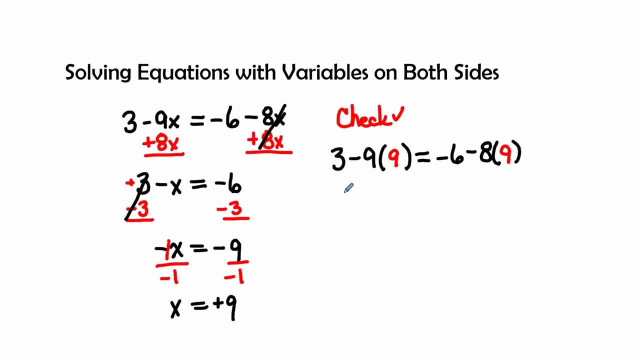 positive 9s. So I have 3 and a negative 9 times 9 is a negative 81. Equals a negative 6 and a negative 8 times 9 is a negative 72. So I see that 3, this is a positive 3. If I don't see a negative symbol in front of it. 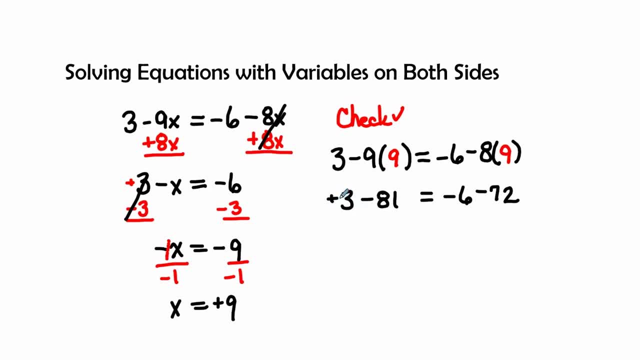 negative sign in front of it, I know it is a positive. So I have a positive 3 and a negative 81. That is going to give me a negative 78. And I have a negative 6 and a negative 72. So I'm going to combine those together. So this: 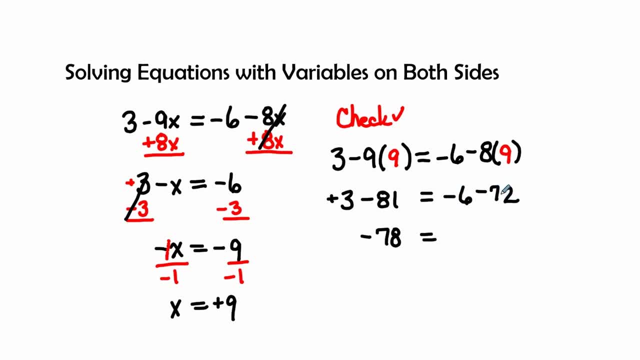 it's just. I'm going to add: I have six negatives here, I have 72 negatives, So together I will have 78 negatives. Wow, this checks, And so we know that our answer of X plus 9 is: or X equals plus 9.. That is our solution. 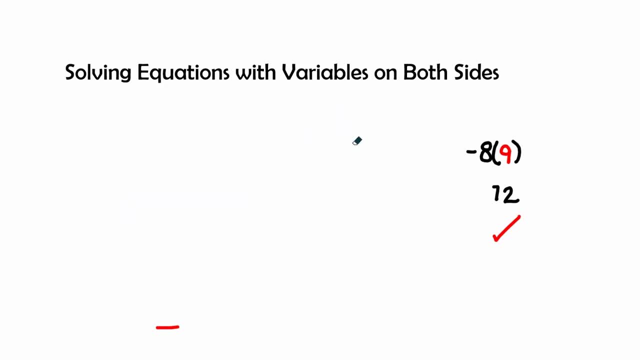 All right, so let's go ahead and erase this. I'm going to. let's do our second problem. Our second problem is going to be negative. 4 plus 5R equals R. So I still have my variables on both sides of the equations. I don't have all my letters on the 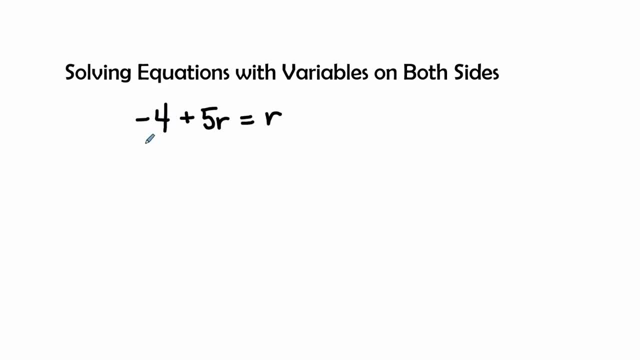 left, So I'm going to end numbers on the right. So let's go ahead and move this negative 4 over to the opposite side of the equation, And how I do that is finding its inverse operation. So the inverse, the negative 4, is a positive 4.. And I'm not going to put that positive 4 under the R. 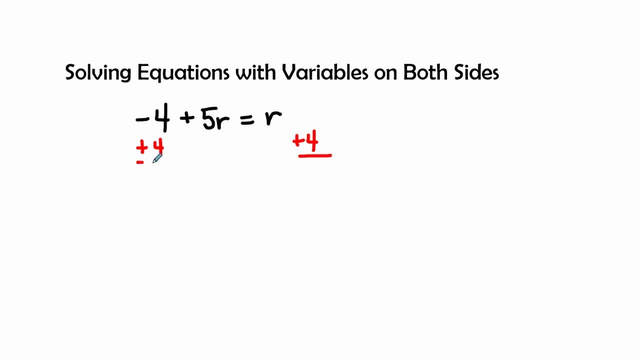 because I'm not going to combine them. I'm going to pretty much imagine if it was R plus 0 right here And now I have my constant terms, that I can do my simple addition. So here we go. A negative 4 and a positive 4 is 0.. I'm going to bring down. 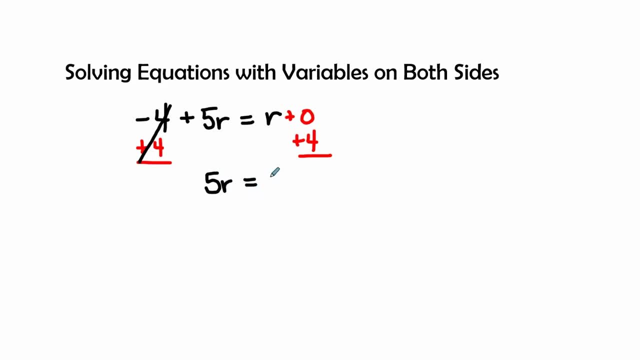 my 5R, keeping my equal signs in line with each other, And I have R plus 0. plus 4 is a plus 4.. Now let's go ahead And in my next step, I'm going to get my variable R, which is a positive R. 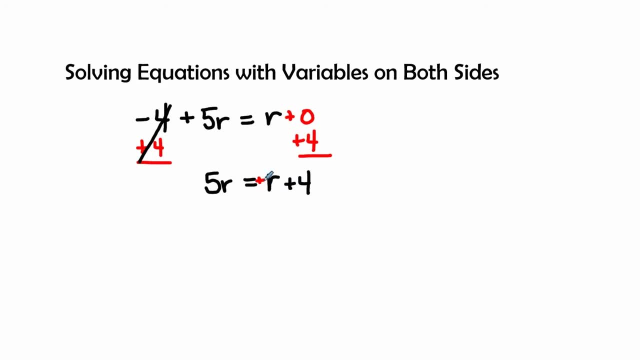 because I don't see a negative symbol in front of that. I know it is positive, And the same thing here. I know that this is going to be a positive 5R, So I'm going to take its inverse- excuse me- as a negative R on both sides. 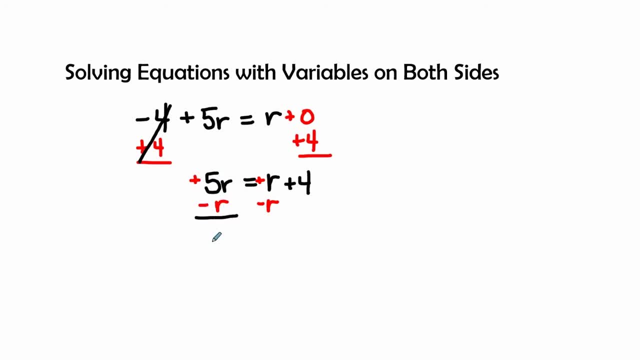 This will give me 5R minus R, results in 4R, And then a positive R and a negative R cancels each other out or equals 0. And then I have a positive 4. Now I ask myself what's attached to this R A 4. How It's attached by multiplication. 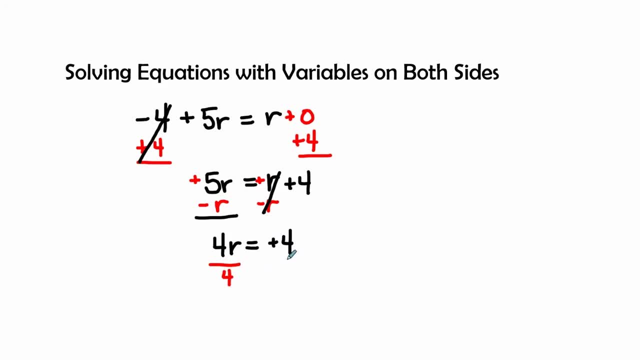 So I'm going to divide both sides by 4.. The opposite of multiplication is division, And what I do on one side, I do on the other side. Now I get 4 divided by 4 gives me R by itself or 1R, And then 4 divided by 4 gives me a positive 1. as my solution. 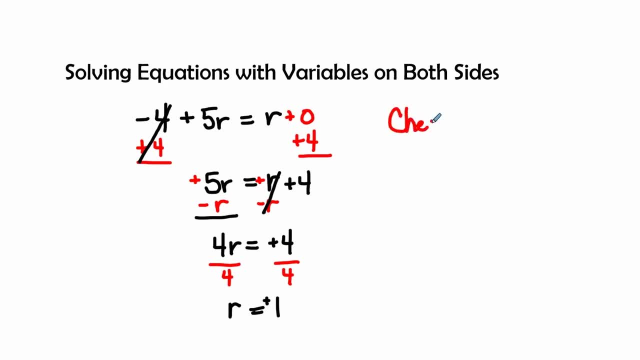 Let's go and check our work. So here we are, We're checking. I'm going to go ahead and write down the equation again, replacing all my variables with parentheses, So I can plug in a positive 1.. And we will see how this all turns out. 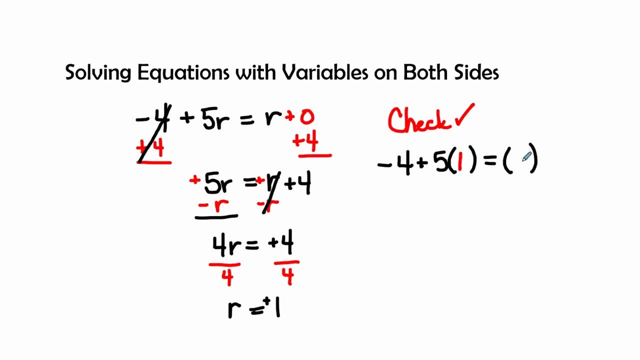 And our goal is to get the exact same number equal to itself at the very end. So here I have: a negative: 4 plus 5 equals 1.. 5 plus a negative 4 is 1.. And sure enough, 1 equals 1.. 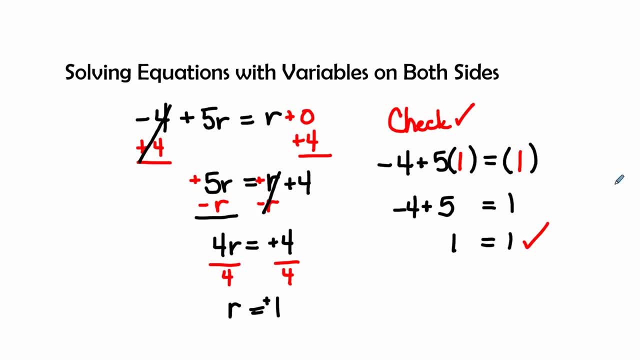 And it checks out. All right. One more example. How are you guys getting this? Are you guys doing OK? So let's go ahead and get rid of everything And let's go ahead and write our third example. This third example is negative. 9 with variable P times the variable P equals 44. 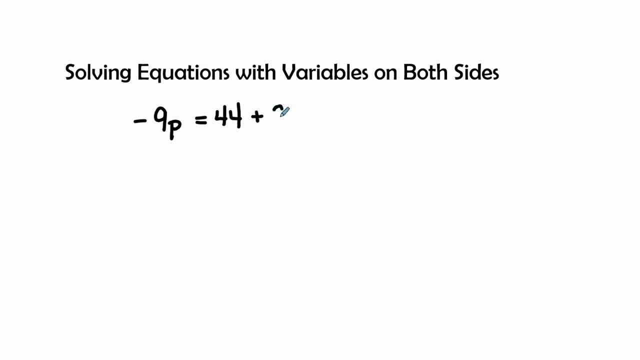 plus 2P. So right away, I see that here's one variable, I have my constant And then I have another variable, So let's move this variable all over to the other side. And how do I do that? Yeah, 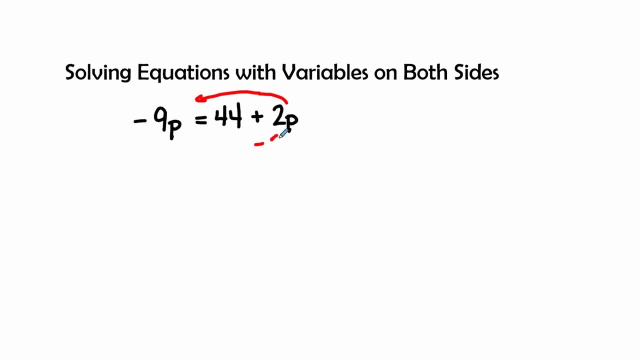 you're right Finding the inverse operation. So I'm going to add a negative 2P to both sides. This gives me a negative 9. P plus a negative 2P, because I'm combining like terms here. So combining means adding them. 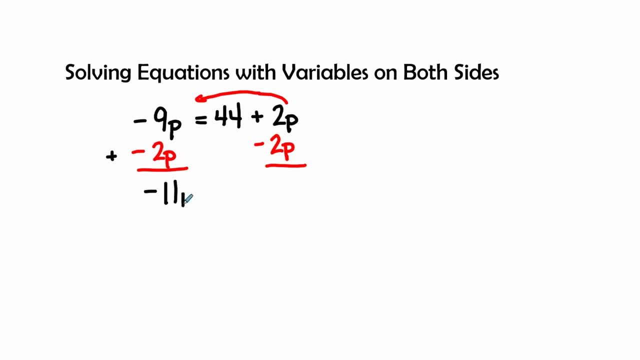 together, So I will have a negative 11P And then I'll bring my 44 down. Then, of course, positive 2P, and a negative 2P gives me zero, And it's no longer on the right hand side when I moved it over. So now I'm going to divide by, because a negative 11,. 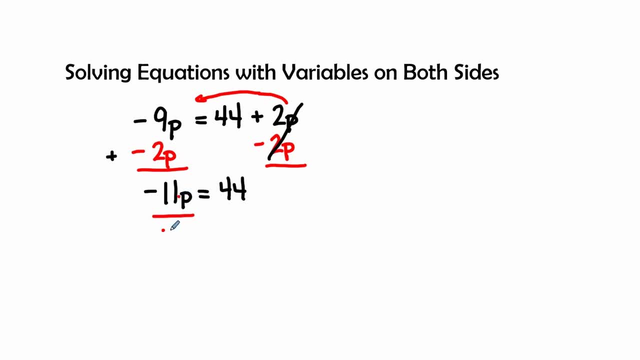 times P. So to get rid of multiplication, I am going to divide by 11 on both sides. Therefore, I have negative 11 divided by a negative. 11 gives me P by itself And I have a positive here. So a positive and a negative is going to give me a negative answer. 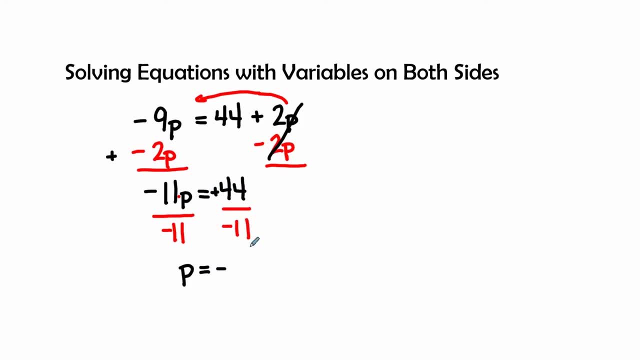 And 44 divided by a negative 11 will give me a negative 4. As an answer. So let's go ahead and check. Whoops, Yeah, let's be a little bit, spell it correctly here. Here we go: Negative 9.. Instead of the P, I'm going to put parentheses for the variable 44 plus 2..